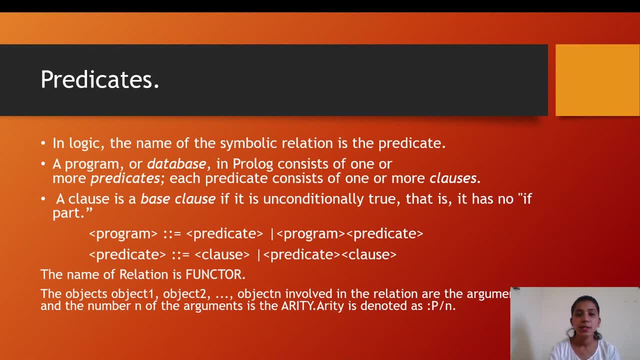 for today's discussion, that is, predicates. What are predicates? In logic, the name of the symbolic relation is a predicate. Predicates are much similar To the functions in our programming languages but they are way different in functioning. A program or database in prologue consists of one or more predicates. Each predicate. 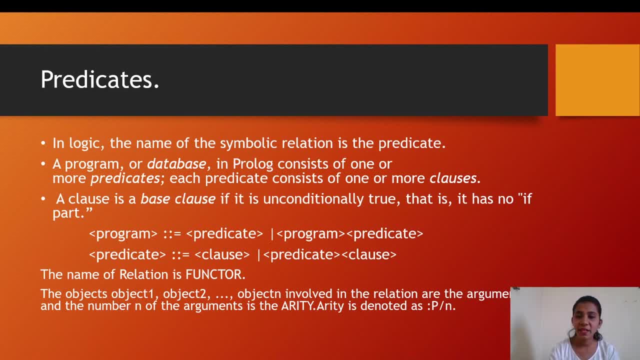 consists of one or more clauses. A clause is a base clause if it is unconditionally true. What is unconditionally true? That is, it has no if part for the program statement. This is a simple syntax for defining a predicate. So let's see how to define a predicate. 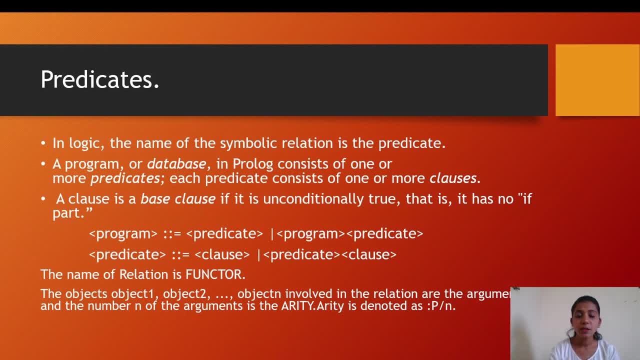 So let's see how to define a predicate. So let's see how to define a predicate: The name of relation is a functor. The name of relation, that is the name of our predicate. Then we have the objects: object1, object2, objectn. involved in the relation are the arguments. 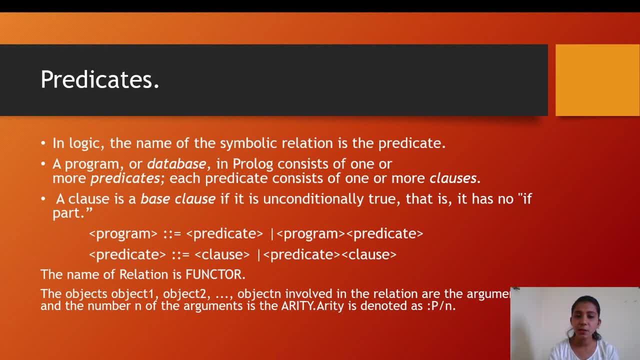 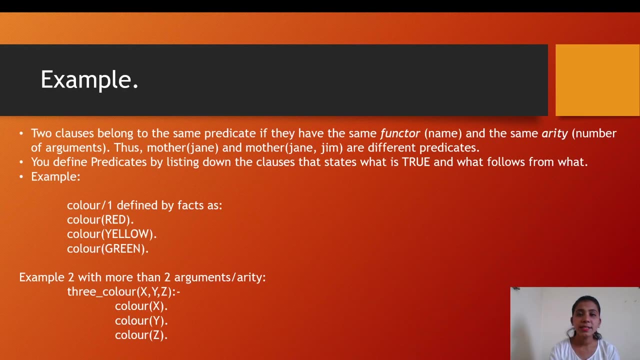 and the number n of the arguments is called the arity. Arity is denoted by p, slash, n. P stands for the name of the predicate and n the number of arguments it can accept. This is a simple example of predicate Before that, two clauses belong to the same predicate. 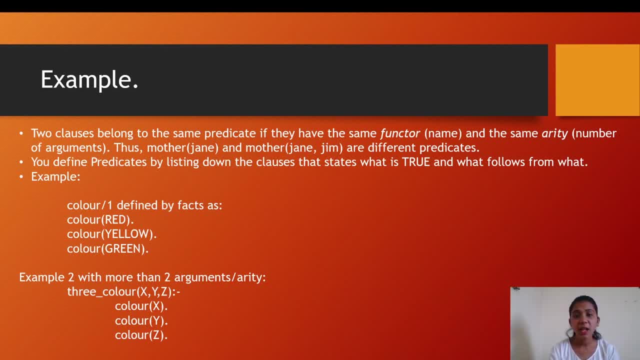 if they have same functor or the same name and the same arity, that is, the number of arguments are also same, Then they belong to the same predicate. That is like, for example, a mother Jane and mother Jane comma Jim. These are the same name predicates but they have different. 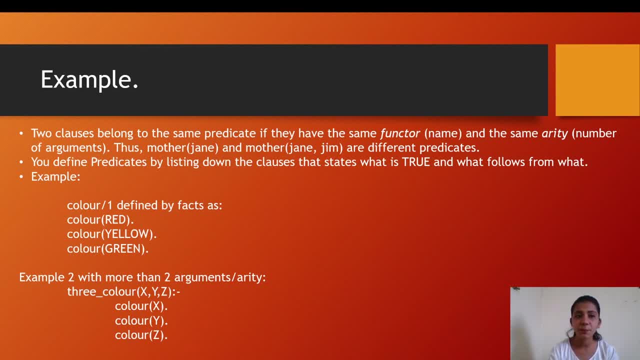 number of arguments. So they belong to the same predicate. So they belong to the same predicate. Next, one define predicates by listing down the clauses that state what is true and what follows from what. Here are some simple examples of predicates: Color 1, defined by Facts as color red, color yellow, color green. These can be read as: 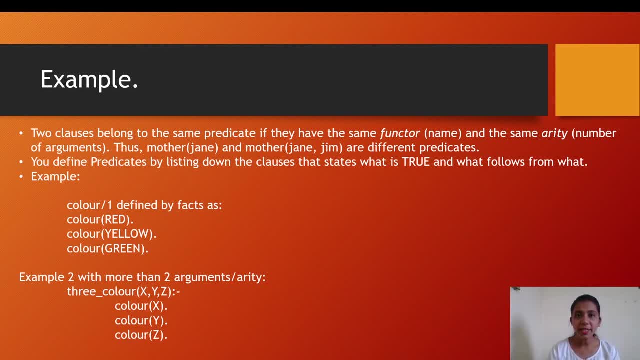 Red is a color, Yellow is a color, Green is a color. There is another example with more than two arguments. this is Arity. This can be defined three color XYZ, which holds when: color X, color Y, color Z. this can be read as: 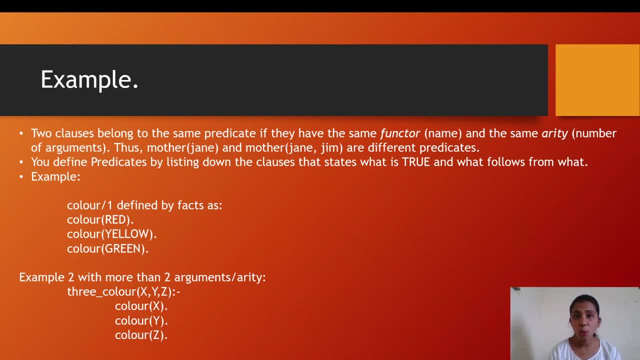 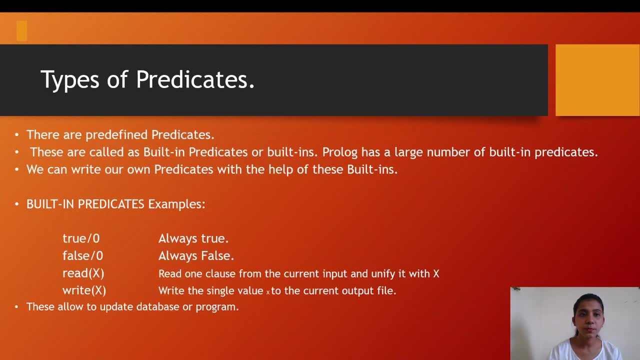 three colors. XYZ holds true only and only if X is a color, Y is a color and Z is a color. then we have types of predicates. there are predefined predicates and there are predicates which we can define as a user. these are called built-in predicates. the predefined predicates are known as: 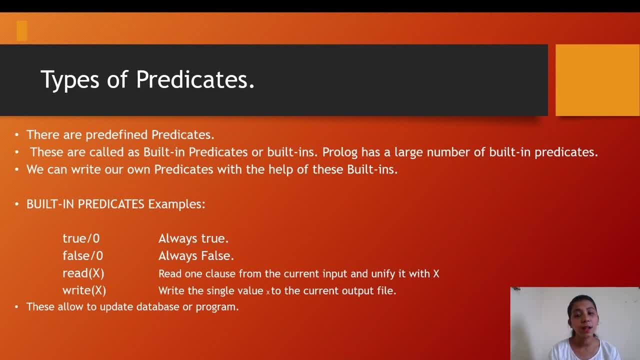 built-in predicates or the built-ins prologue has a large number of built-in predicates. we can write our own predicates with the help of these predefined built-in predicates. these are the examples for built-in predicates that must be present in your prologue library: true slash zero, which is always 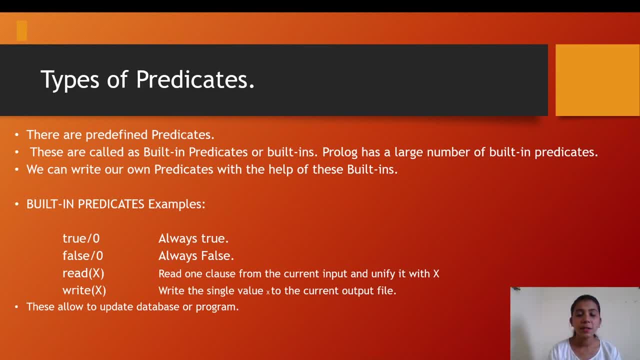 true, false. slash zero, which is always false. read X, which means read one clause from the current input and unify it with the current input, and unify it with X. then we have another write X predicate, which means write the single value of X to the current output file. these were some of 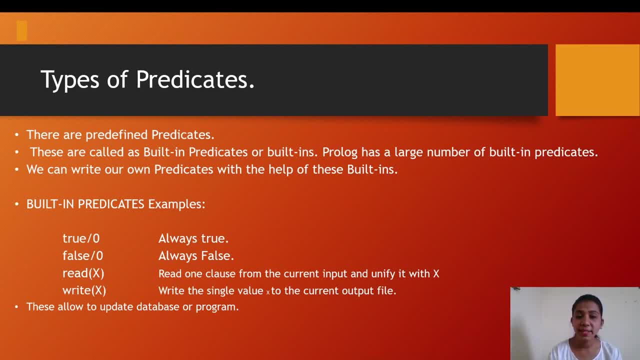 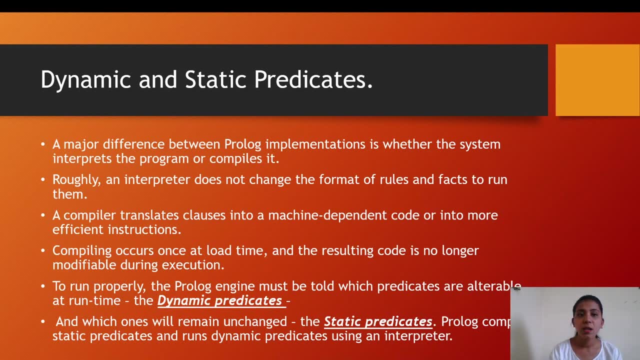 the examples of built-in predicates. these allow to update, our update a database or a program. then we have dynamic or static predicates. a major difference between prologue implementation is whether the system interprets the program or compiles it. this means prologue either can be interpreted or can be compiled roughly. an interpreter does not change the 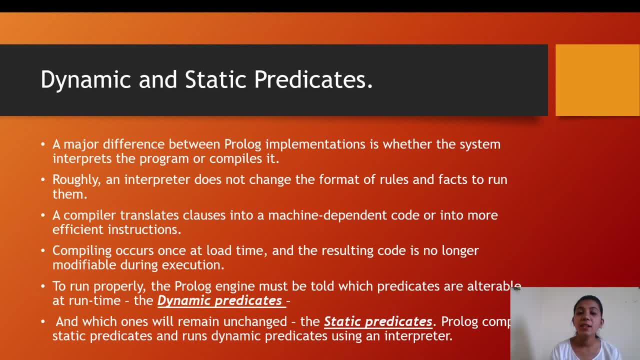 format of rules and facts to run them, a compiler translates the clauses into machine dependent code or into one more, one or more efficient instructions. compiling occurs once at load time and the resulting code is no longer modifiable during the execution. now to run the prologue in to run a program. 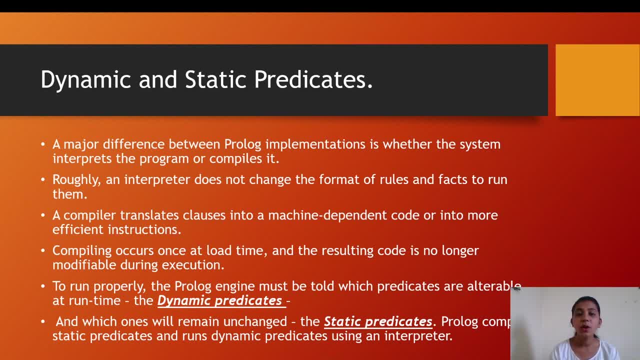 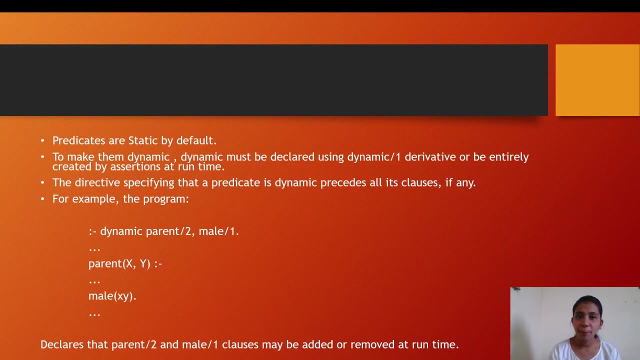 nicely and efficiently and properly. the prologue engine must be told which predicates are alterable at the runtime. the alterable ones are called the dynamic predicates and the ones which will remain unchanged are known as static predicates. prologue compiles static predicates and runs dynamic predicates using an interpreter. predicates are static by default. to make